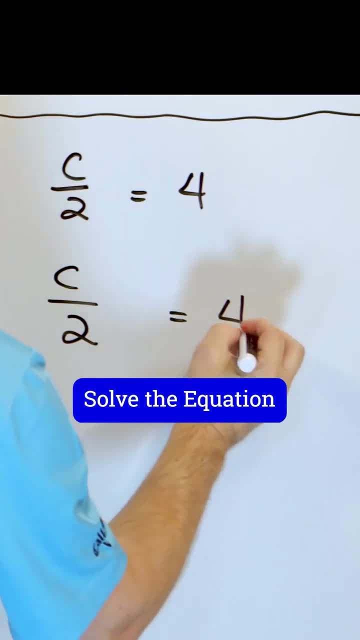 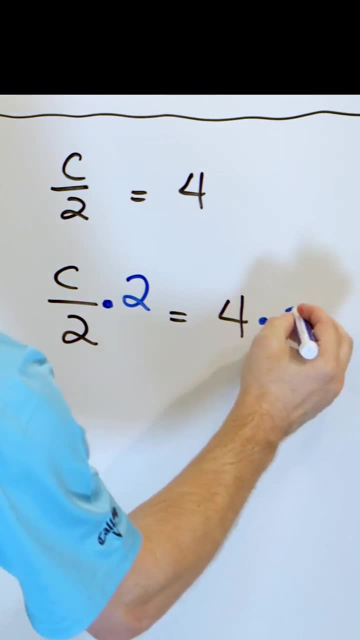 Let's rewrite the problem: C over 2 is equal to 4.. Now what do we do here? We're dividing by 2.. We want to do the opposite, So we're going to multiply by 2 on both sides, And this 2,. 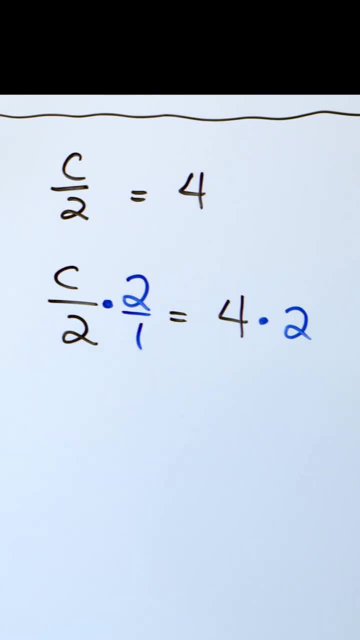 we're going to just write it as 2 over 1 to help us visualize what's happening Now: the 2 on the top and the bottom. because these fractions are multiplied, we can cancel them, And then, on the left-hand side, we're going to be just left with C. Well, it's really C divided by 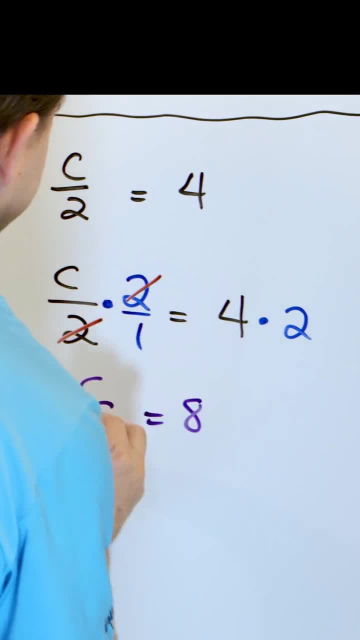 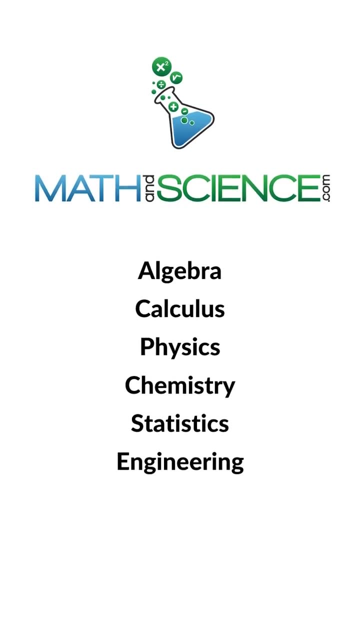 1,, but that's just C. And then 4 times 2 is 8. And so the answer is 8.. And you can check by putting 8 in here: 8 divided by 2 is 4. And so that's the right answer. Learn anything at mathandsciencecom. 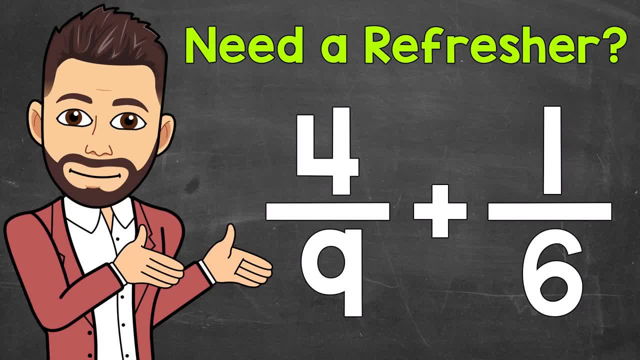 Welcome to Math with Mr J. In this video, I'm going to go through a quick review of adding fractions. If it's been a while and you need a quick refresher, this should be helpful Whether you're in middle school, high school, college, continuing your education as an adult. or just learned this recently. Really, no matter where you're at. here are a couple of examples to help you out. Let's jump into number 1, where we have 3 7ths plus 2 7ths. Now, when we add fractions, we have to have a common denominator. 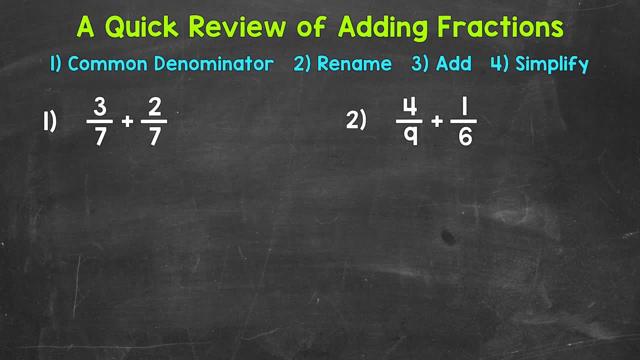 So we always look to see if our denominators are the same. If they're the same, we can add. So in the case of number 1, we have a 7 and a 7 for our denominator, So we have a common denominator right away. 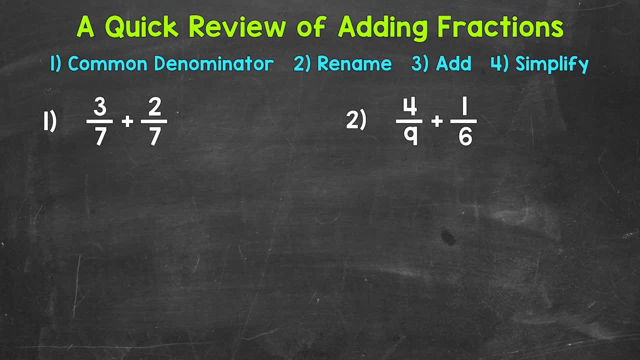 That means we can add. So we add the numerator: 3 plus 2 is 5.. So this is going to equal 5.. And then we keep our denominator the same: 5, 7ths is our answer. We can always look to see if we can simplify. 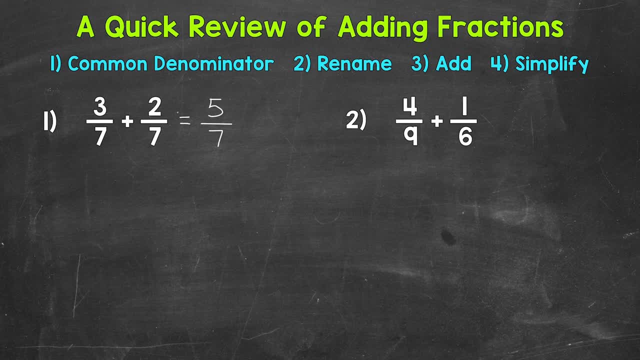 The only common factor between 5 and 7 is 1.. So we are done. 5 7ths is in simplest form and our final answer- Again for number 1, we had a common denominator, So we were able to add right away: